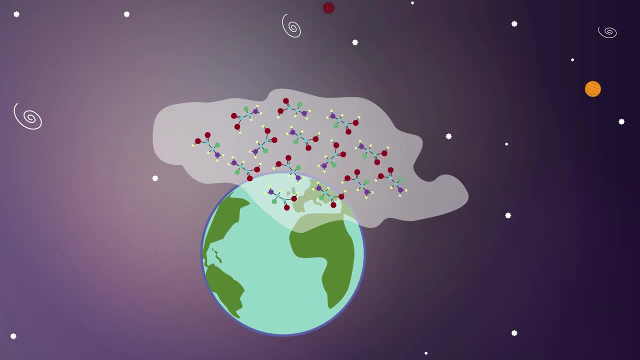 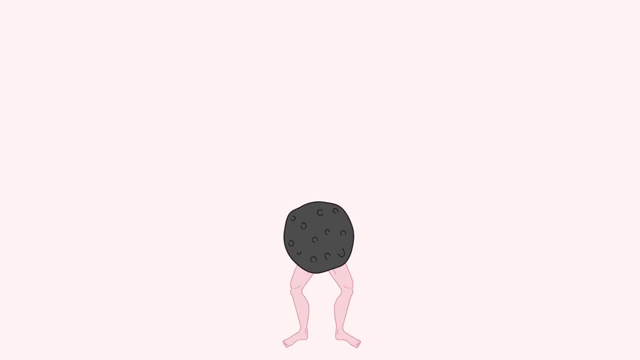 observation of prebiotic chemicals present in interstellar clouds, It seems pretty evident that some raw materials, such as amino acids, must have fallen on earth to help kickstart life. Some other researchers have proposed that it's not just organic substances but even small organisms like bacteria that could evolve in space on grains of matter. 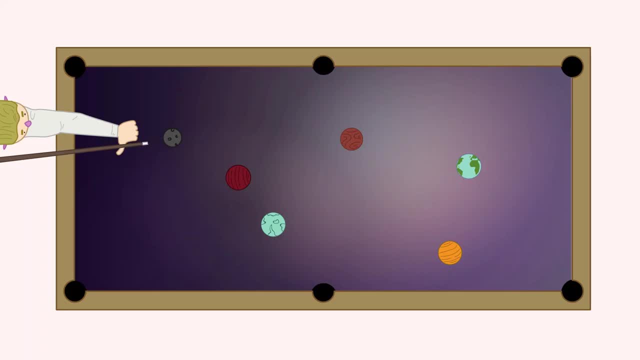 and then be brought to the earth or have an impact in common. An alternate version of this is known as spore spores. This theory is known as directed panspermia. This modern idea of panspermia theory originates from the observation of prebiotic chemicals present in interstellar clouds, It seems. 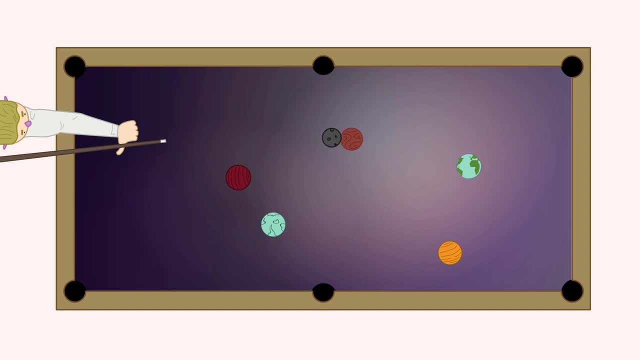 pretty evident that some raw materials, such as amino acids, must have fallen on earth to help kickstart life. This theory is known as ballistic panspermia. This essentially involves rock from one planet being blasted into space by a colliding comet and then travelling to another planet. The fact that 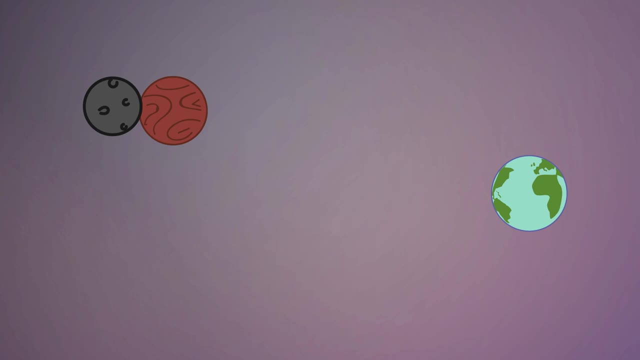 we have discovered meteorites from Mars here on earth might mean we all originated from aliens. 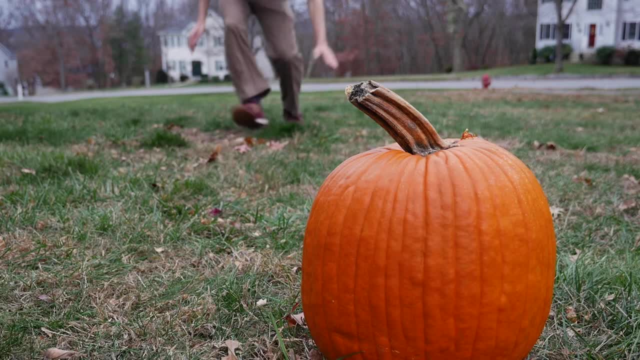 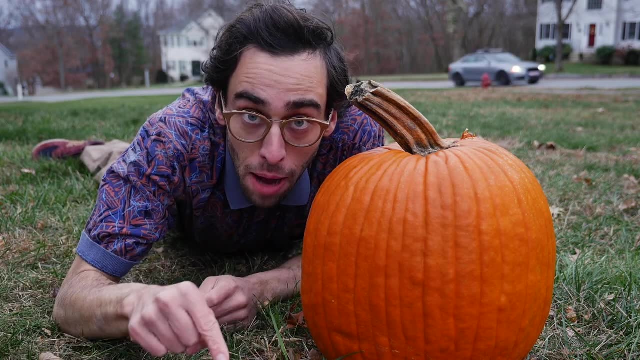 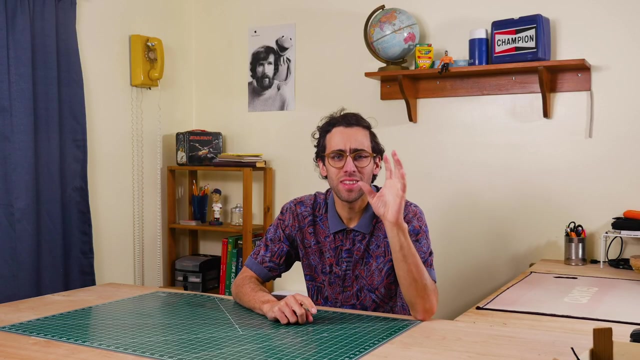 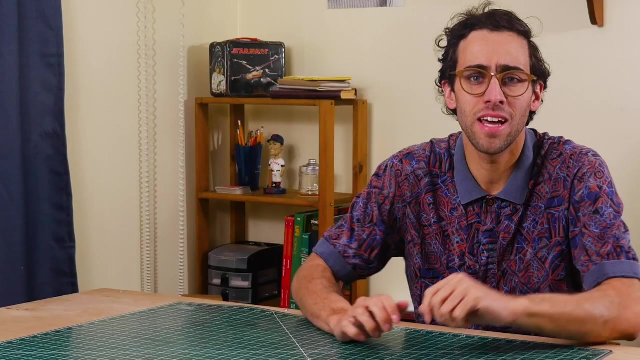 Would you believe me if I told you that everything in the universe, from this pumpkin to a popsicle, is made from just 118 different ingredients? No, I'm serious, It's true. Everything living and nonliving in the entire universe is made from some combination of the 118 elements. 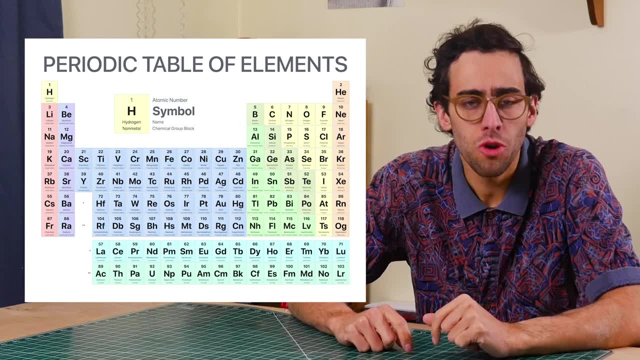 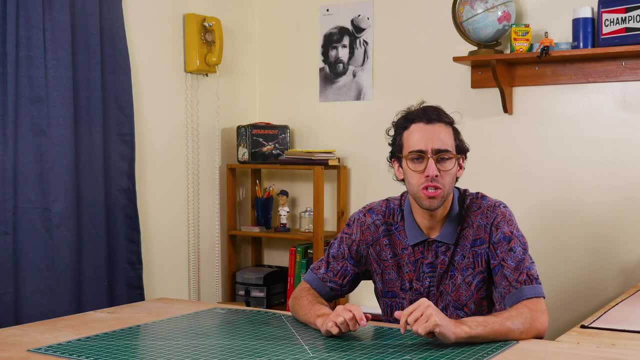 on this chart right here called the periodic table of elements. Here we have oxygen and hydrogen, carbon and nitrogen. All of these ingredients are called elements. Now, you may have heard this word before element, But what does it mean? And what are compounds? 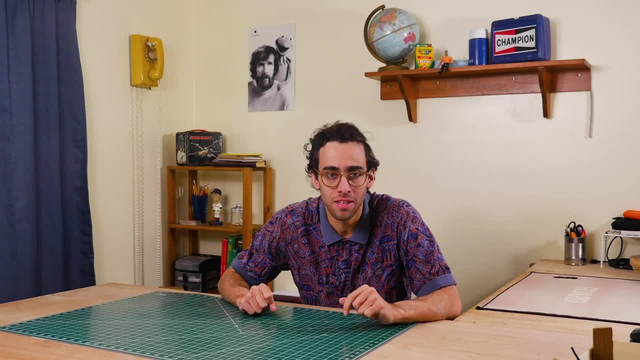 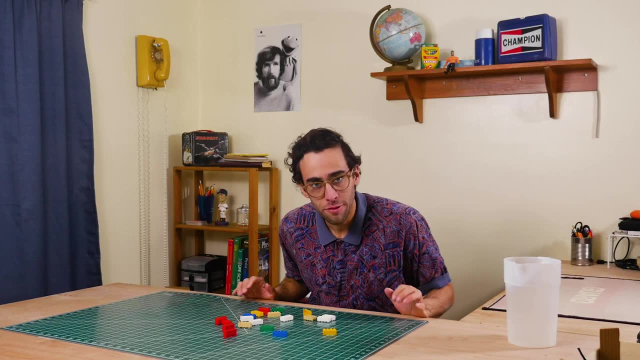 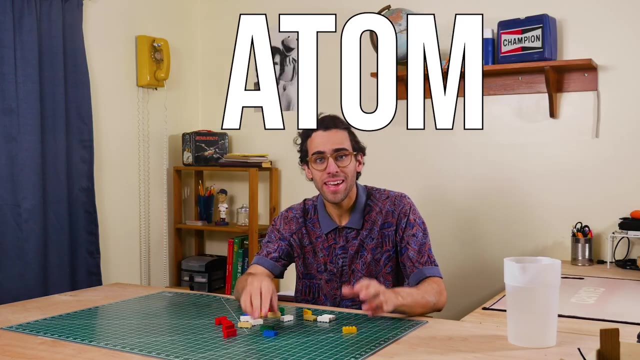 and mixtures. Well, I have an easy way to help you understand it. And we use Legos. So we have all of these different Lego bricks And we'll pretend that each Lego brick is an individual atom. okay, Just like how Lego bricks are the building. 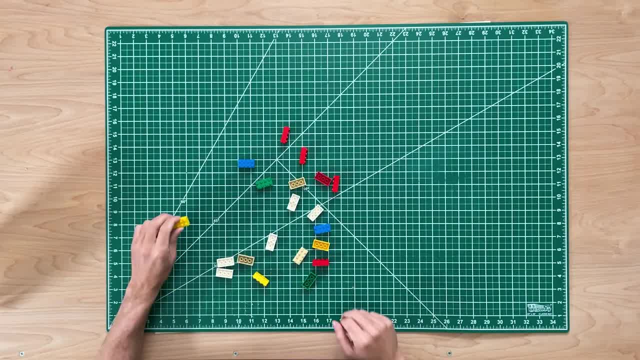 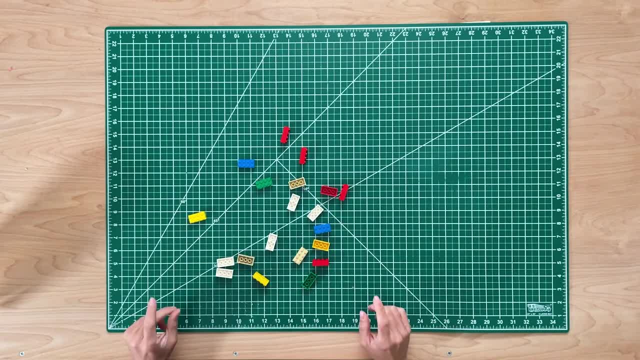 blocks of a building. Lego bricks are the building blocks of a building And Lego bricks are the building blocks of a building. And Lego bricks are the building blocks of a building And Lego bricks are the building blocks for awesome Lego creations. These atoms are the building blocks for everything in the universe. Seriously, And notice how.